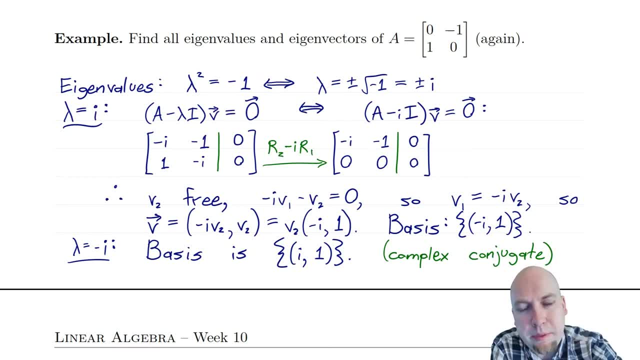 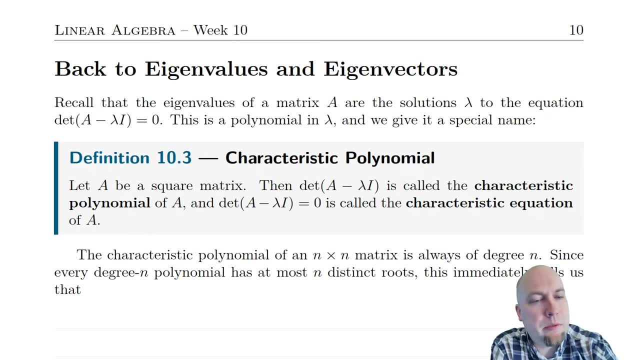 size of the matrix. The matrix is two by two. The degree of this polynomial equation is two. Okay, and that's not a coincidence, This always happens. Okay, so this polynomial is something that we call the characteristic polynomial. This determinant of a minus lambda i is the characteristic polynomial. 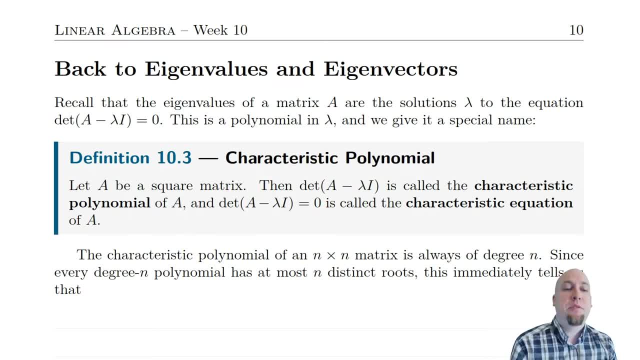 And the equation determinant of a minus lambda i equals zero. that's the characteristic equation. Okay, and the reason that it's always a polynomial of degree n is well, suppose they've got an n by n matrix. You're computing determinants of this thing here and remember from last week we have: 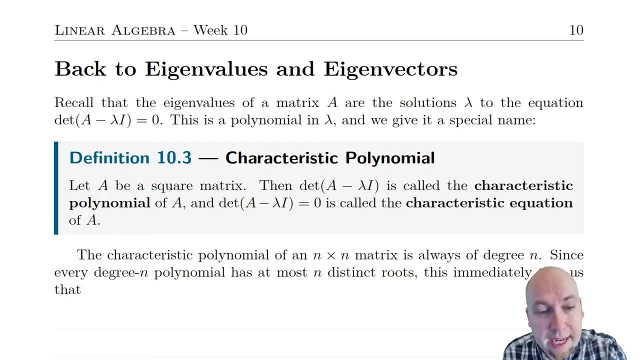 explicit formulas for this determinant. Okay, and if you use those explicit formulas, you always get exactly this polynomial that we're talking about. Because, well, think about how these explicit formulas are constructed: They're constructed from cofactor. expansion: They're constructed from cofactor. 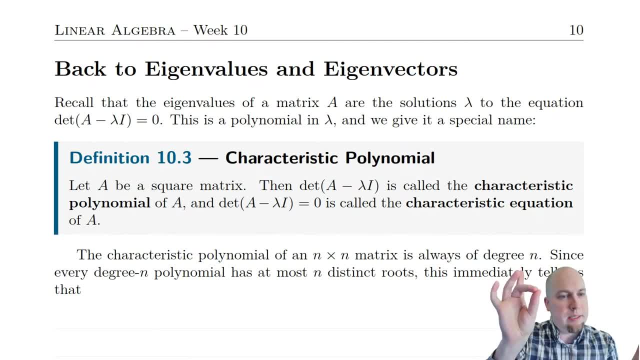 expansions. And when you construct something out of cofactor expansions like this, if the matrix is n by n, what you're doing is you're adding up and subtracting a whole bunch of terms, and each one of those terms is a product of n entries, of a minus lambda, i. Okay. and if you're multiplying? 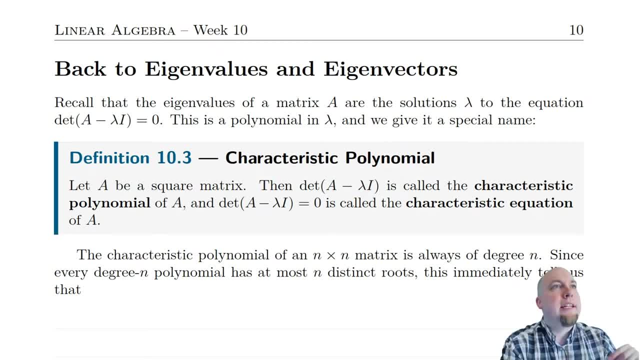 together n entries from a minus lambda i. well, each of those things that you're going to multiply together has either zero or one lambdas in it. So when you multiply together n of them, they have zero lambdas in it. So it's going to be a polynomial of degree less than or equal to n, And furthermore, 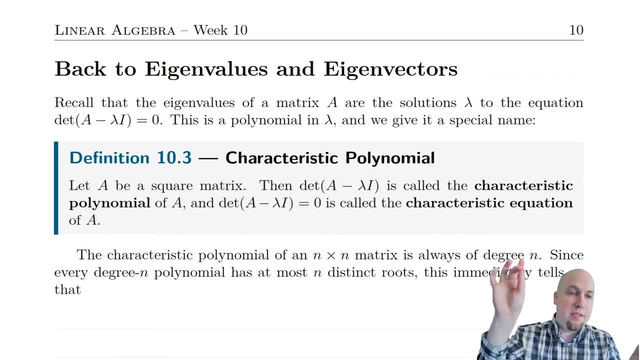 on the diagonal, you have exactly n lambdas. Okay, and that term. when you multiply it together, all the diagonal entries. that is one of the terms in the determinant. Okay, in these cofactor expansions. Okay, so this thing here it really is. it's always a polynomial in lambda and it always has. 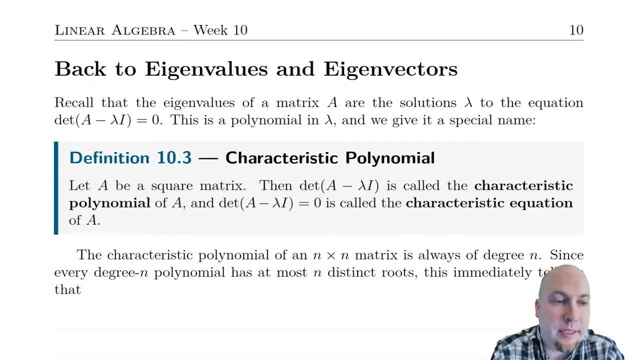 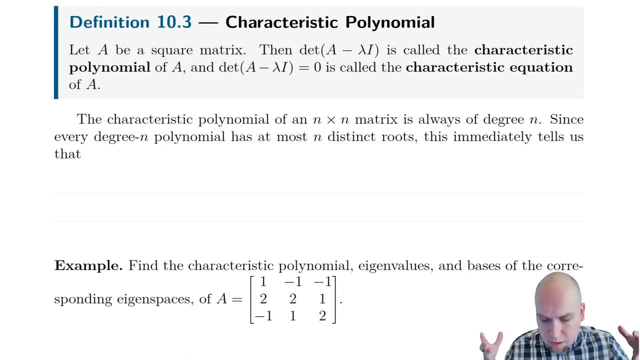 degree exactly equal to n, the size of the matrix. Okay, and this observation is useful because we know lots of things about polynomials. So now that we know we get eigenvalues from polynomials, well right away we're going to know lots of things about eigenvalues as well. So, for example, 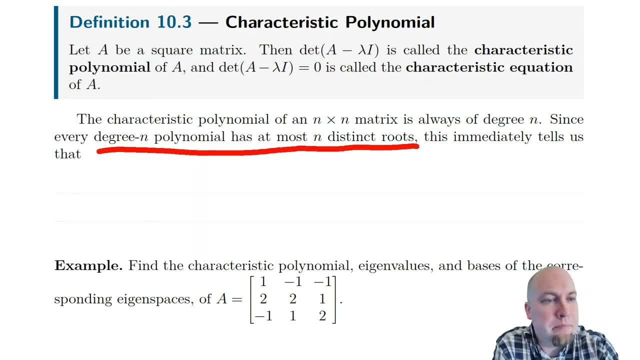 we know that every degree n polynomial has at most n distinct roots, which immediately tells us, if we just string these facts together, that if you have an n by n matrix, it has at most n eigenvalues. Okay, an n by n matrix, like a two by two matrix, is never going to have three. 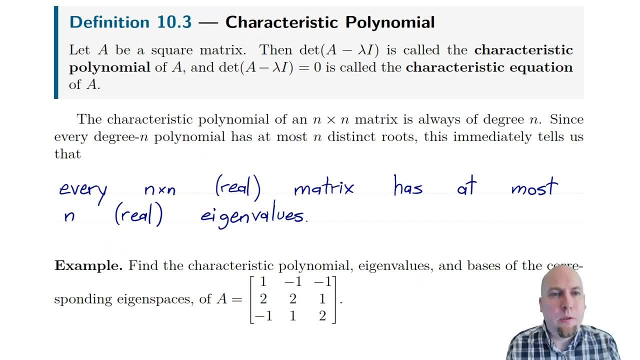 eigenvalues. It's never going to have four eigenvalues. It'll either have n by n, or it'll have n by n, Or it'll have zero, one or two. always Okay, because we know that these eigenvalues they come. 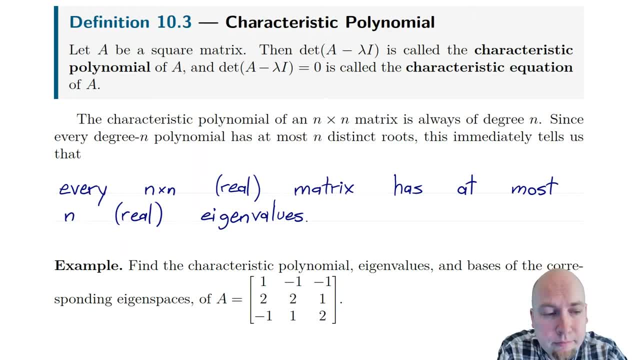 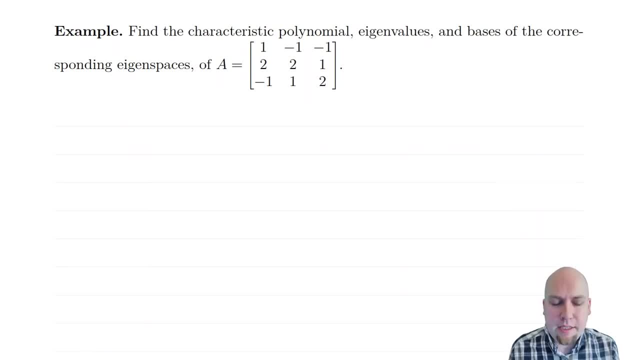 from a polynomial equation of degree two. All right, so let's go through another example of computing eigenvalues and eigenvectors. now that we have this in mind, now that we understand eigenvalues a little bit better, Okay, so here we've got a three by three matrix. Okay, so we 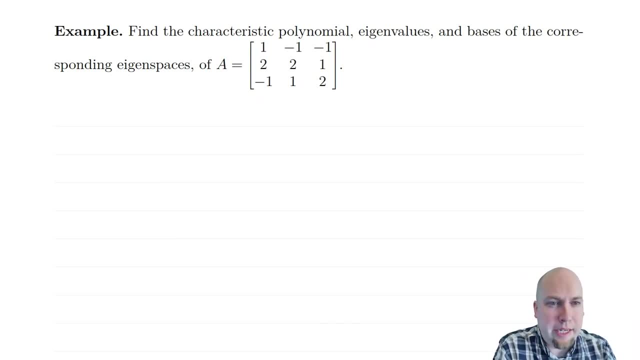 know right away we're going to find at most three eigenvalues. All right, let's actually find them. Okay. so step one, find the eigenvalues, then we'll do eigenvectors later. So to find eigenvalues, set determinant of a minus lambda i equal to zero, which just means you take this matrix. 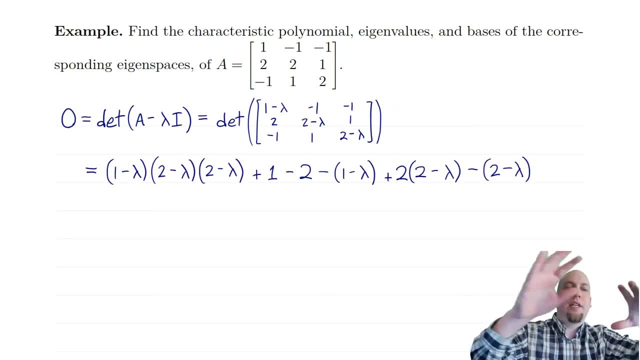 subtract lambda off of the diagonal. Okay, then we use our explicit formulas for the determinant to expand out that determinant there, right? So it's going to be the product of the forward diagonal, which is this first term here, then the product of the next wrapping around forward. 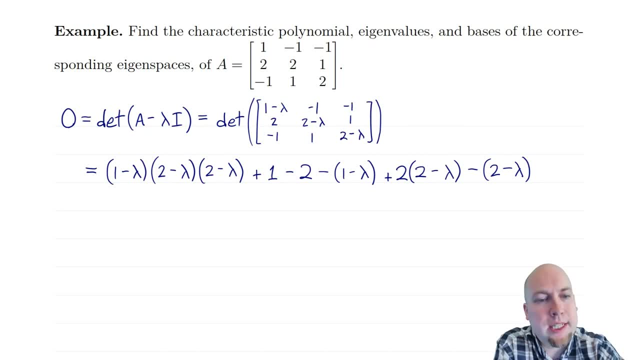 diagonal, which is this plus one, and the next wrapping around forward diagonal is the minus two, and then the three backward diagonals as well, also wrapping around. Okay, and those gives us those three negative terms there. Okay, now remember, our goal is to get this polynomial completely factored, so that we can see what its 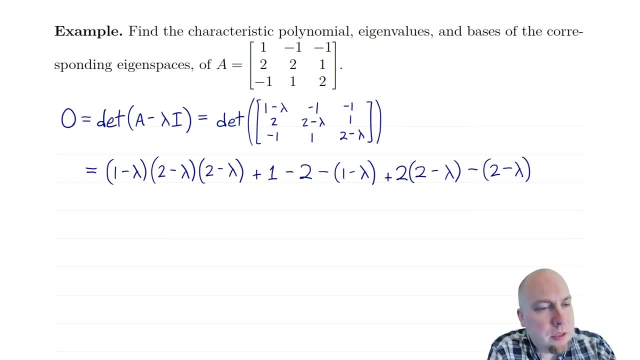 roots are, because those roots are the eigenvalues. So what I'm going to do first is I'm going to simplify these terms over here. Okay, I got two times something minus that thing, so I'm going to start off by, you know, canceling out the extra multiple there, so that I've just got a single two. 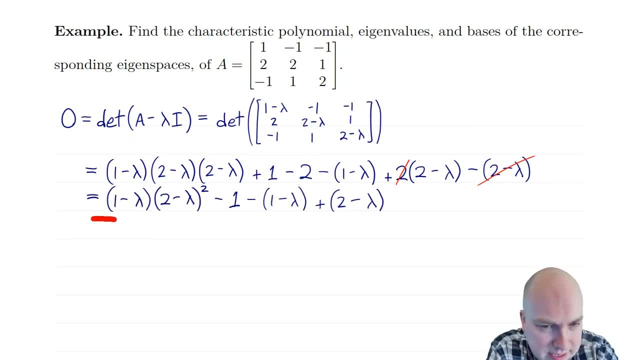 minus lambda, Okay, and when that simplifies down, it simplifies to this Notice. I've combined these two terms here into a two minus lambda squared, Okay. and now if you look at these terms over here really carefully, you'll notice that actually the two minus lambda squared is the lambda squared. 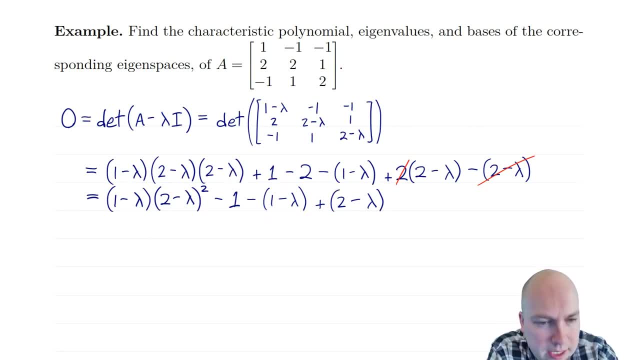 Notice that actually, every single one of them cancels out with each other. We've got a negative negative lambda, and we've got a plus negative lambda. Okay, we've got a minus one minus one plus two. Those all cancel out with each other and you're just left with this first term here. 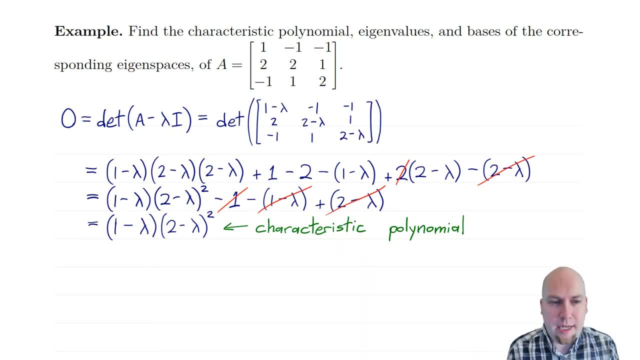 Okay, which is already factored. It saved us the trouble of having to factor anything just by noticing that everything over here canceled out with itself. Okay, so then this: this is the characteristic polynomial and, furthermore, it's the factored form of the characteristic polynomial. 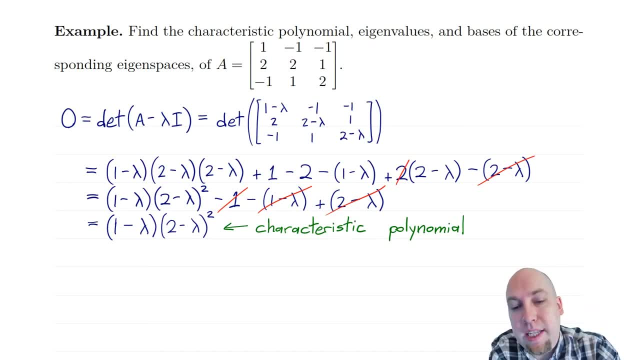 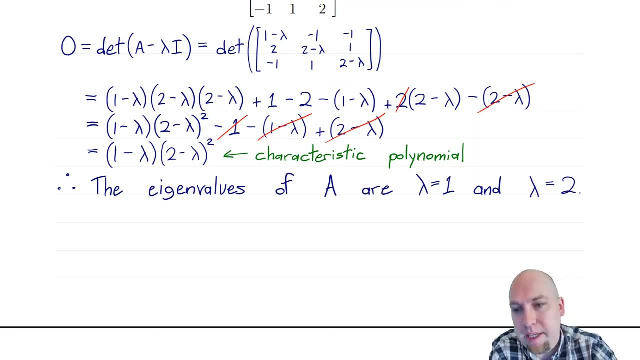 that makes it easy to see what the eigenvalues are. So we're going to start off by calculating what the eigenvalues are. So the eigenvalues are just the roots. In other words, the eigenvalues are one and two. Okay, so those are the only eigenvalues of the matrix, And I mean this is. 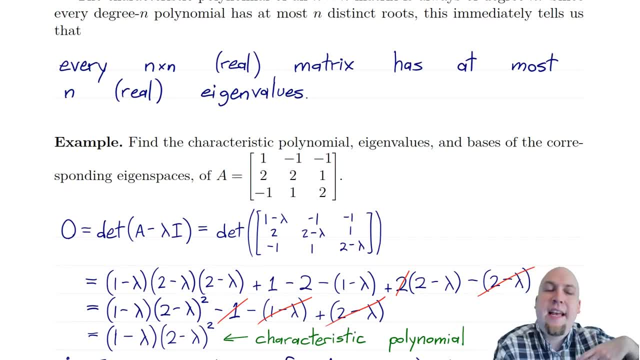 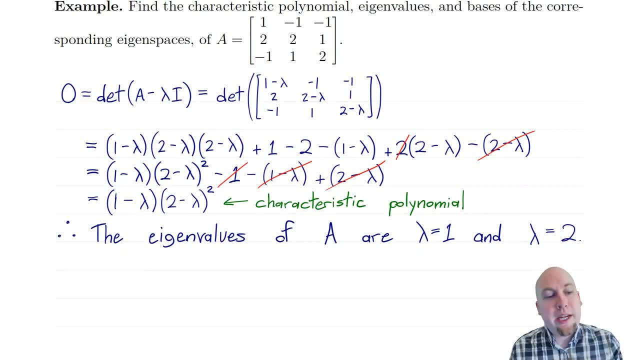 consistent with what we said before. It's a three by three matrix. It has, at most, three eigenvalues- Okay, here it has two eigenvalues, two distinct eigenvalues- Okay, great. So we know the eigenvalues of the matrix one and two. We know the characteristic polynomial of the matrix, So all that's left is 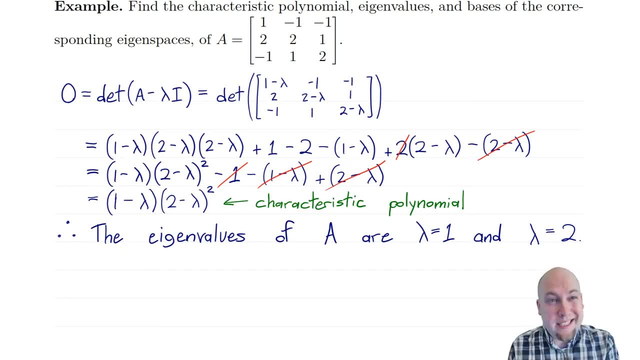 find the eigenvectors of the matrix And, in particular, we're going to find bases of the matrix. Okay, so what do we do? Well, we set up the linear system that we always set up to find eigenvectors. Okay, you start off with one eigenvalue at a time. So lambda equals one is as: 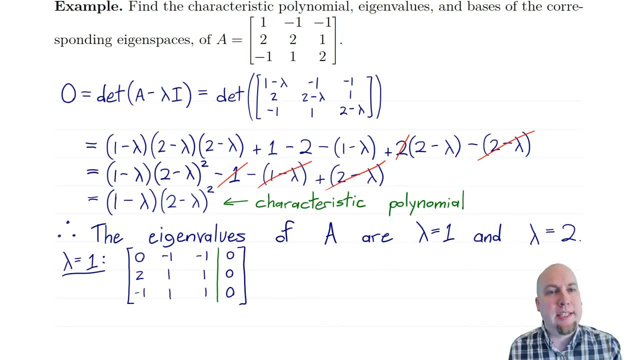 good a starting point as any. And you subtract lambda off of the diagonal of A, So we're going to subtract one from the diagonal entry. So one's going to become zero, two will become one, and two will become one And we get zero one one down the diagonal. now, Okay, so this is A minus lambda. I. 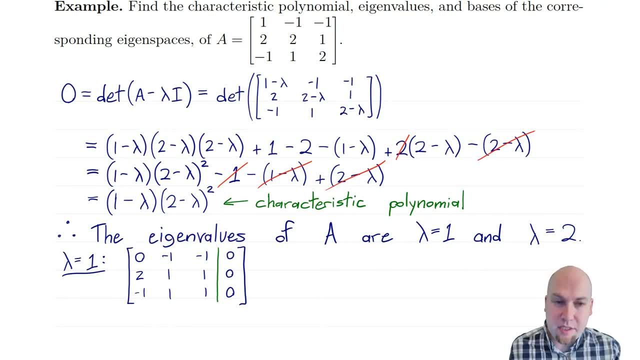 and augment with zeros on the right hand side. That's the linear system that you solve: to find eigenvectors. Okay, and then just go ahead and solve that linear system. Okay, do Gauss-Jordan elimination, bring it all the way down to reduced row echelon form, and you're going to get this. So I've skipped. 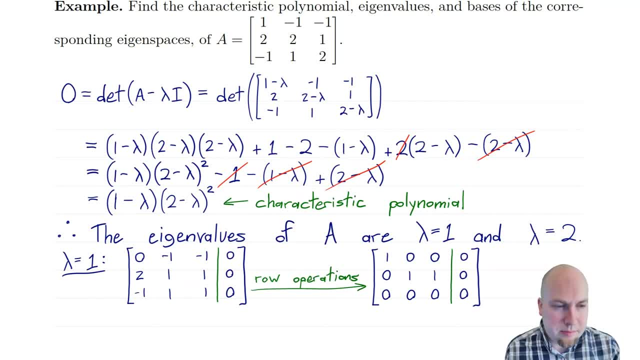 over the row operations. You can try that on your own. You know how to solve linear systems at this point. Okay, and now we look at this reduced row echelon form and we see: ah, there's a leading entry in that first column, There's a leading entry in that second column, but there's no. 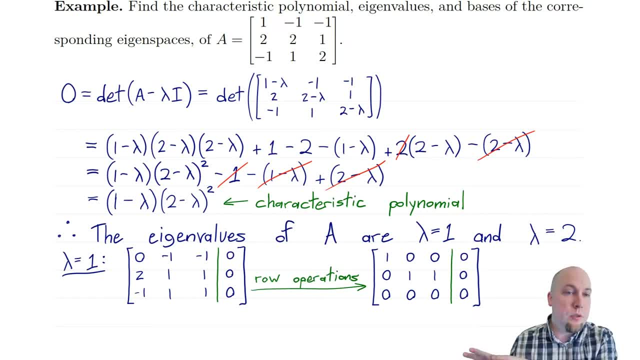 leading entry in the third column. So that means v1 and v2, the first two entries of the eigenvectors. those are leading, whereas v3, the third entry of that eigenvector, it's free. It can be anything it wants to be. Okay. so v1, v2 are leading, but v3 is free. 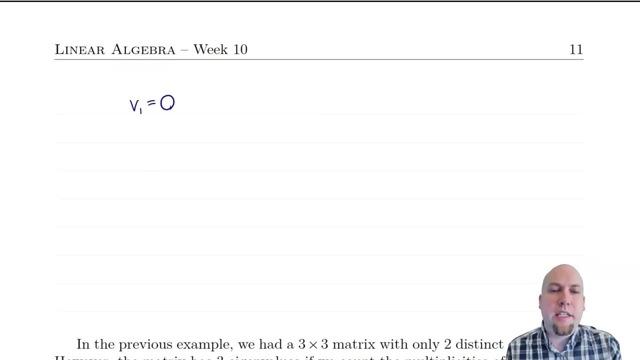 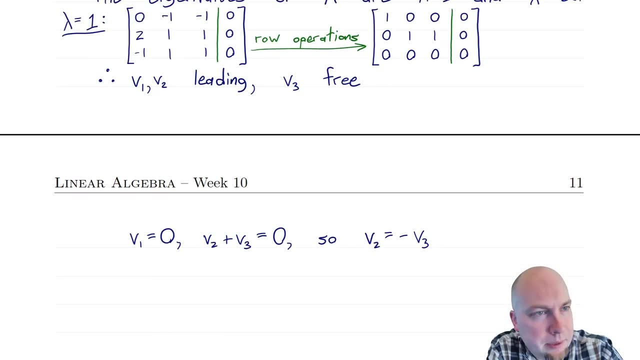 Okay, and then what we can do is we can look at this reduced row echelon form and figure out what those entries of the eigenvector have to be as well. Okay, so I'm going to scroll back up here just a little bit. If we look at this first row- remember that's an equation and what this tells: 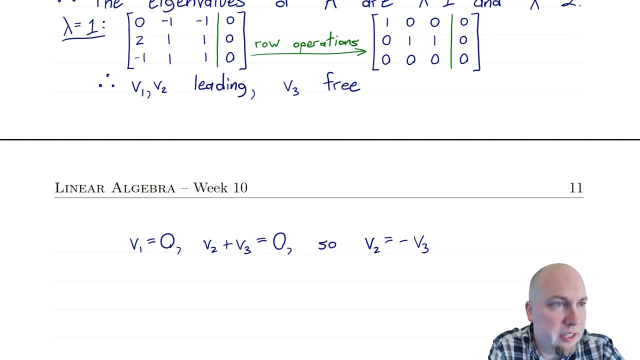 us is 1 times v1 plus 0, v2 plus 0, v3 equals 0.. Okay, so that's v1 equals 0.. The second equation tells us: 0v1 plus v2 plus v3 equals 0.. So that's our second equation And for any equation involving 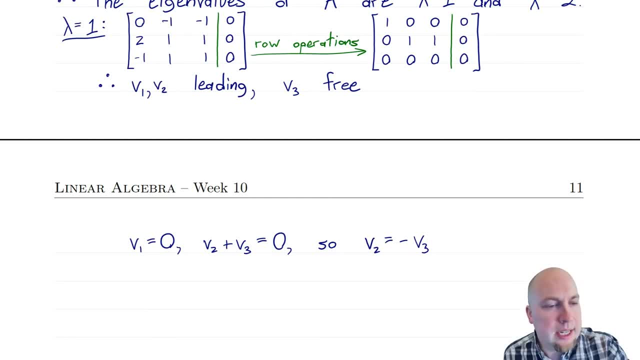 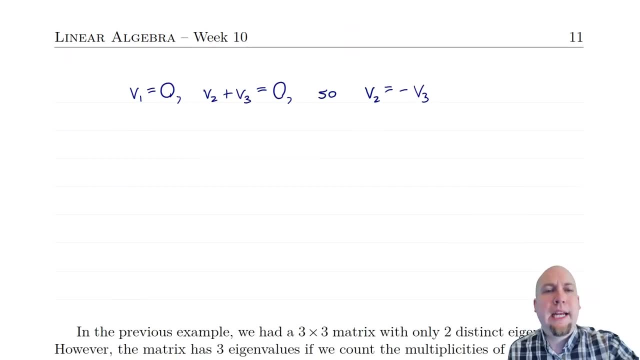 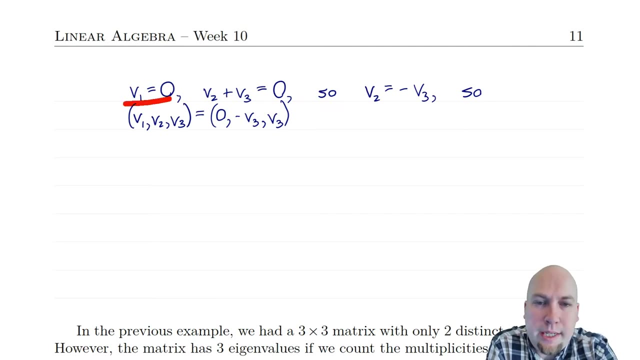 a free variable. just rearrange it so that it's leading variable in terms of the free variables. Okay, so rearrange this equation to get: v2 equals minus v3.. Okay, and then you can stick this into vector form. Okay, you just say: hey, v1, v2, v3, what does that equal? Well, what was v1 equal? 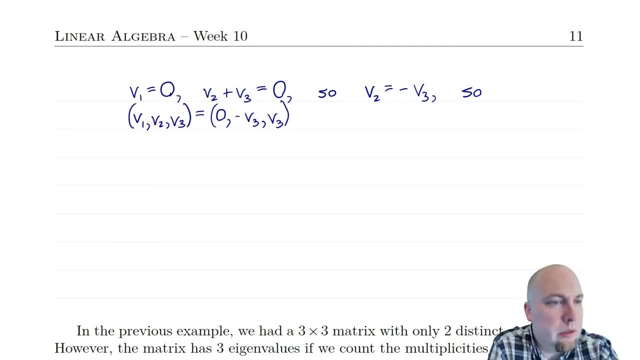 It equals 0.. So I put that in the first slot. And then what is v2 equal? Well, it equals minus v3.. so I put that in the second slot. and then what is v3 equal? well, v3 is free, so it just equals itself. 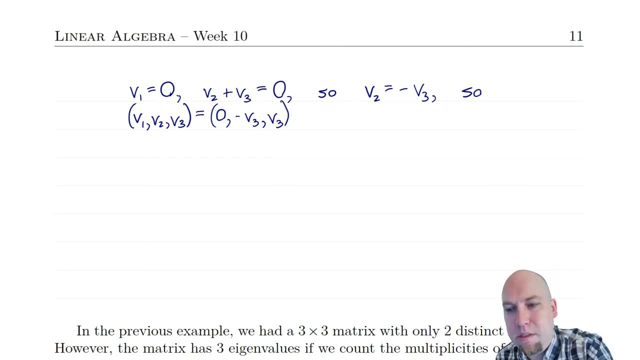 it can be anything it wants, to be okay. and then, as always with the eigenvector calculations, you can pull the free variables out at the end of the day. pull the v3 out, in this case, and you're going to get 0 minus 1 and 1 left over, so all of your eigenvectors corresponding to lambda equals. 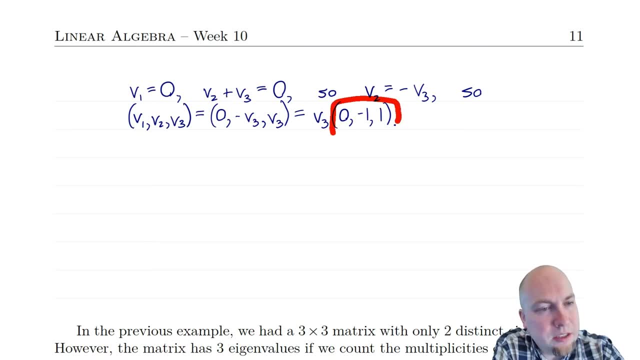 1 are multiples of this vector here 0 minus 1, 1. so in other words, this vector 0 minus 1, 1 forms a basis of that one-dimensional eigen space. all right, let's do the other the same thing. for the other eigenvalue lambda equals 2, so this time we've subtracted 2 off of the 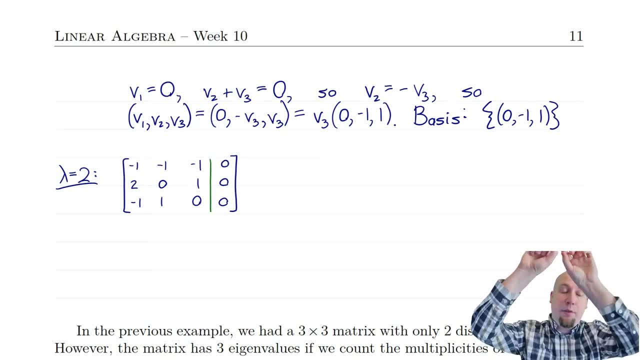 diagonal of a. so the diagonal used to be like for a itself, it was 2 1, 1. well, I'll subtract 2 off of each of those, and now the diagonal is minus 1 0, 0. and again you do your row reduction magic. 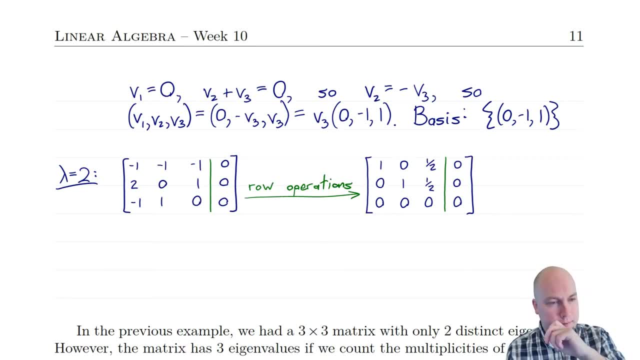 bring that all the way down to reduce row echelon form and you get this matrix over here and we see something very similar happens here to what happened on the previous page. first, two columns each have a leading entry, so v1 and v2 are leading. third column has no leading. 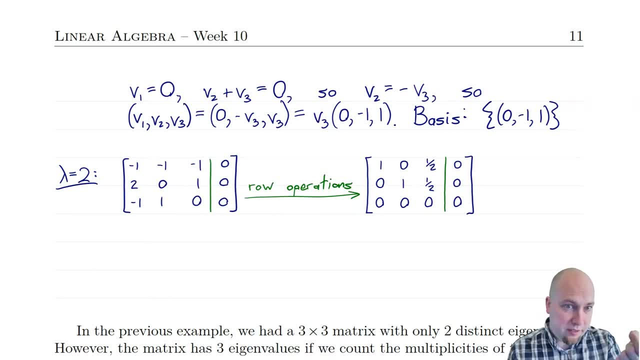 entry. okay. so the third variable, v3, the third entry in your eigenvector is free. okay, it can be anything it wants to be. okay, so v1, v2 are leading. v3 is free because there's no leading entry in that third column. okay, and then just write down what these equations mean. okay, this. 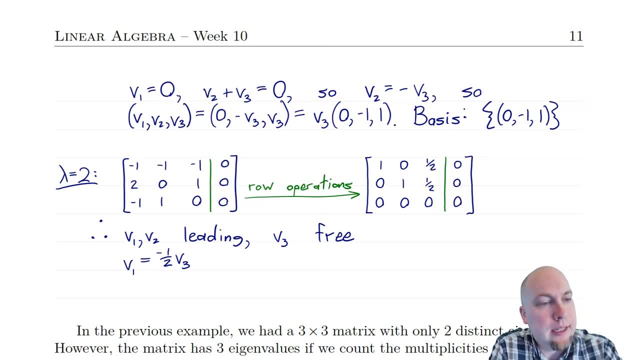 tells us that v1 plus a half v3 equals zero, and rearrange that so that it's leading variable in terms of free variables. okay, so leading equals something involving free. okay. and similarly, the second row that tells us 1 v2 plus one half of v3 equals zero, we'll just rearrange so that the 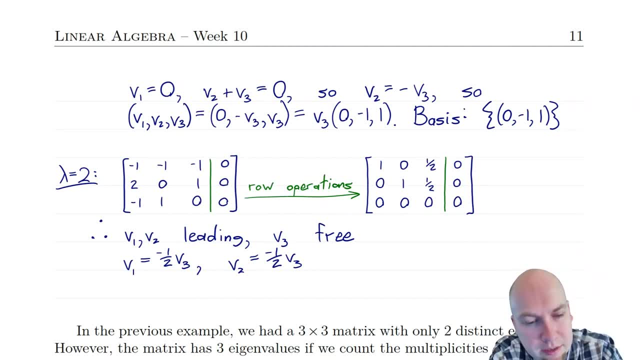 leading variables on one side of the equation, free variables are all on the other side of the equation and you just get this: bring them the one half, v3, over to the right hand side. okay, and then what's that tell you? well, if you put in vector form, it tells us that v1, v2, v3 equals. well was. 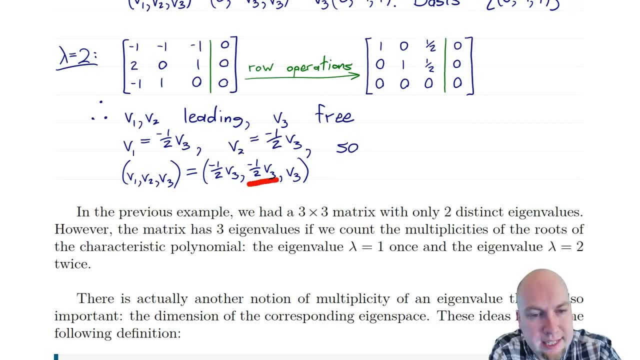 v2 equals minus half a three. was v2 equal? it equals minus half a three. and what's b3 equal? it's free, it just equals itself. and then you can factor the v3 out of everything and you're left with, well, the eigenvectors. they're multiples of minus a half, minus a half one, in other words. 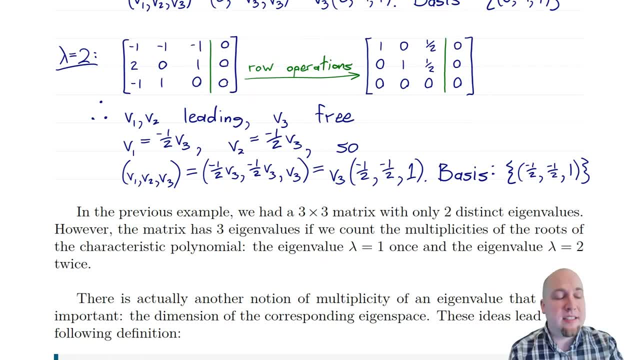 the single vector. here again, it forms an eigens, a basis of the eigenspace, of that one dimensional eigenspace, even okay. so I wanna try to unpack a couple things that occurred in this example here. okay, a three by three matrix that only had two distinct eigenvalues, So it had the eigenvalue one and it. 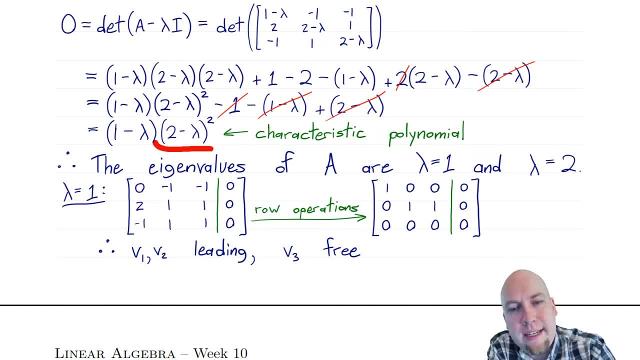 had the eigenvalue two, But this eigenvalue two, in a sense it occurred twice. This characteristic polynomial- here is lambda, one as a root, here is lambda equals two as a root, but it occurs again. In other words, if you sort of write out this polynomial sort of in long form instead of using 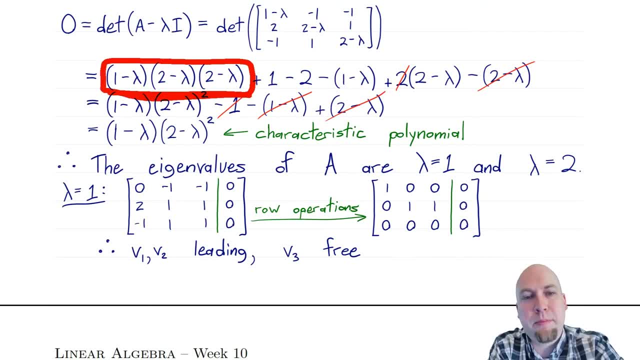 squared up here. you just write out each linear term multiplied by each other linear term, you'll get this expression up here: One minus lambda, times two minus lambda, times two minus lambda, And you can see that two minus lambda is occurring twice. In other words, lambda equals two. 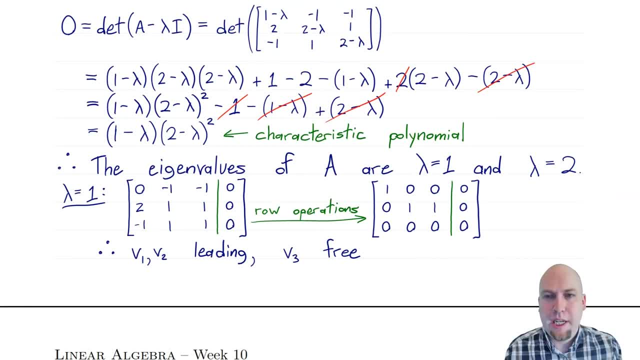 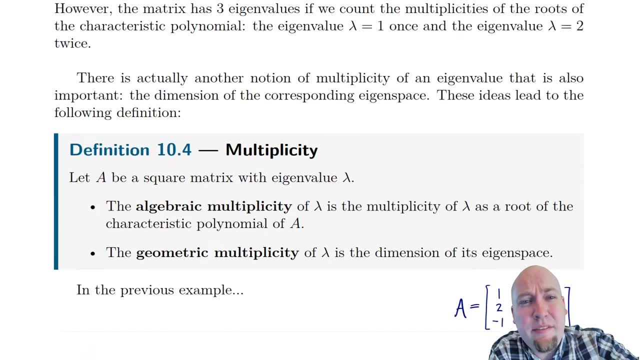 is sort of occurring twice as an eigenvalue And we give a name to this idea of an eigenvalue occurring multiple times as a root of the characteristic polynomial. In other words, this idea of an eigenvalue occurring multiple times as an eigenvalue of a matrix, We call it. 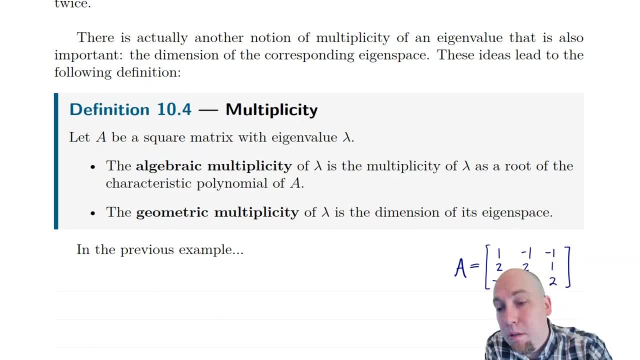 the multiplicity of that eigenvalue And, in particular, occurring multiple times as a root of the characteristic polynomial, We call that the algebraic multiplicity of that eigenvalue. Okay, so the algebraic multiplicity of an eigenvalue, lambda, it's just the multiplicity of lambda as a root of the. 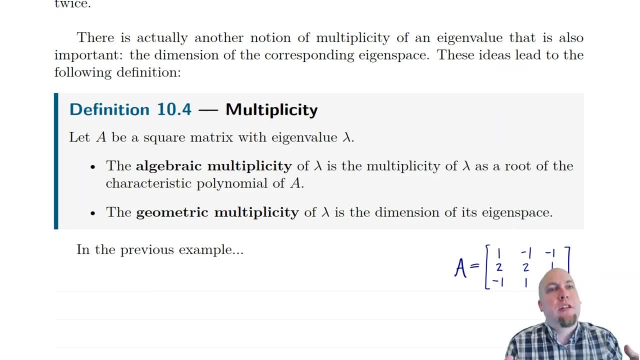 characteristic polynomial. In other words, it's the number of times it occurs as a root of that characteristic polynomial. It's the number of times that that linear factor occurs as a factor. If you completely factor that polynomial, how many times does lambda minus that particular eigenvalue? 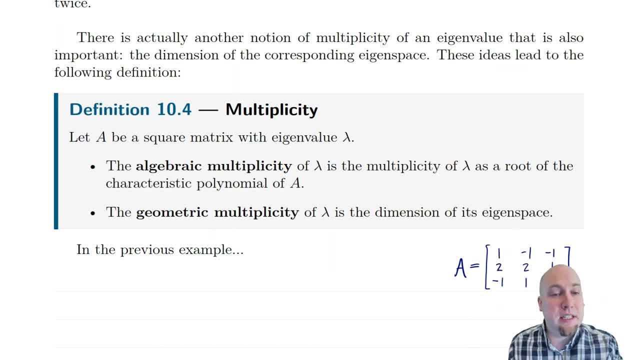 occur as a factor there. Okay, what is the exponent of that factor? That's the algebraic multiplicity. Okay, there's another, slightly different notion of multiplicity as well, though. Okay, we call the geometric multiplicity. Well, that's the dimension of the eigenspace associated. 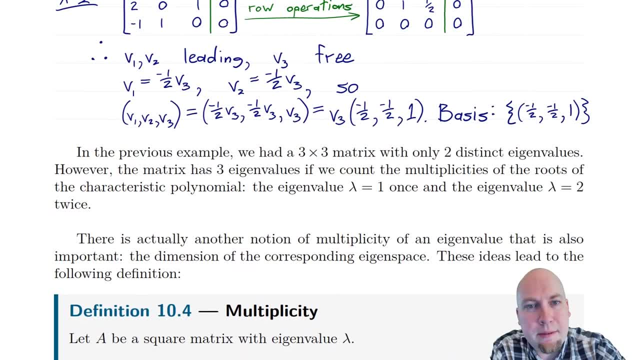 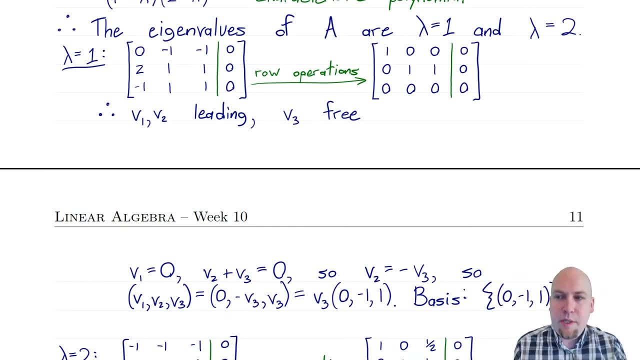 with that eigenvalue, Okay. so if I just scroll back up to this example that we just went through, okay for lambda equals one to compute what the geometric multiplicity of lambda equals one is, we just look at this basis of the eigenspace corresponding to lambda equals one And we see 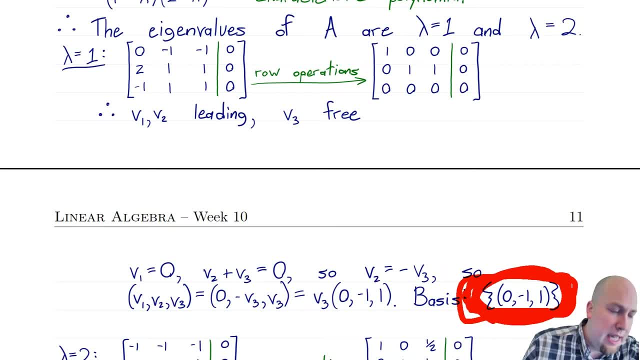 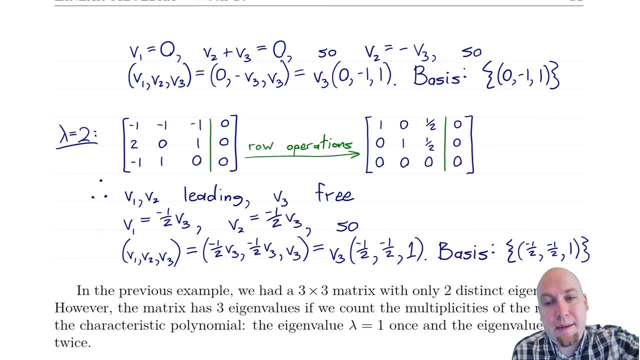 well, how many vectors are in that basis? Well, there's exactly one vector in that basis, So that eigenspace is one-dimensional. Geometric multiplicity is one, Okay. similarly, for lambda equals two. well, here's a basis of the corresponding eigenspace. It only has one vector. 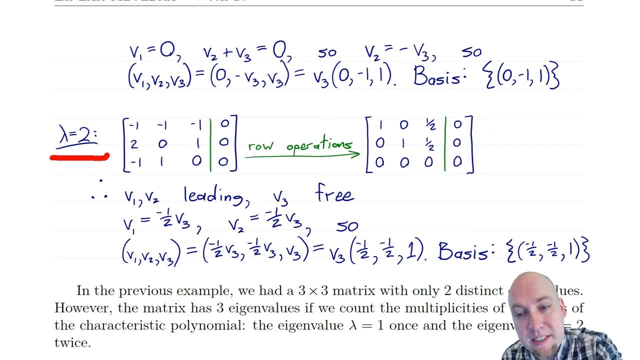 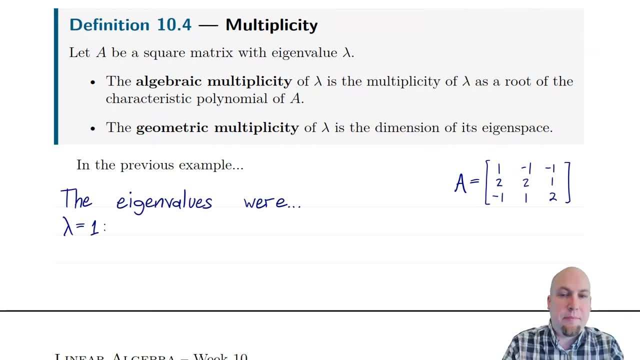 so that eigenspace is one-dimensional. So the geometric multiplicity of lambda equals two is also one. Okay, so let's write this all down, Okay, in the previous example, so this matrix that we talked about, the eigenvalues of just a second ago, the eigenvalues were lambda equals. 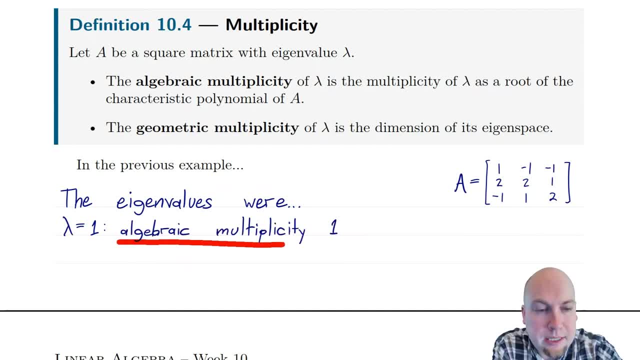 one and lambda equals two. For lambda equals one, the algebraic multiplicity was one, because the lambda minus one term. well, that only occurred as a factor in the characteristic polynomial. just once Lambda equals one was just a root once, And the geometric multiplicity was also. 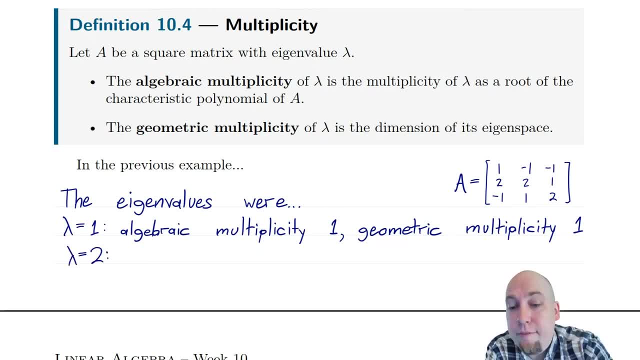 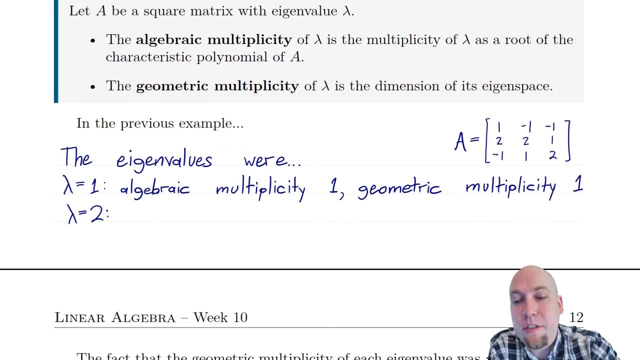 one. okay, because the eigenspace was one-dimensional. For lambda equals two. so, like, every different eigenvalue gets its own algebraic multiplicity and geometric multiplicity for lambda equals two. the algebraic multiplicity this time was two because, remember, lambda equals. 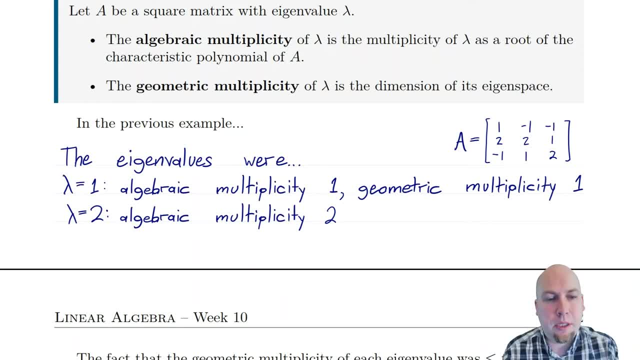 two or two minus lambda. that occurred as a factor in the characteristic polynomial. so the algebraic multiplicity was two. Okay, so the algebraic multiplicity was two. The geometric multiplicity was still one because its eigenspace was still one-dimensional. 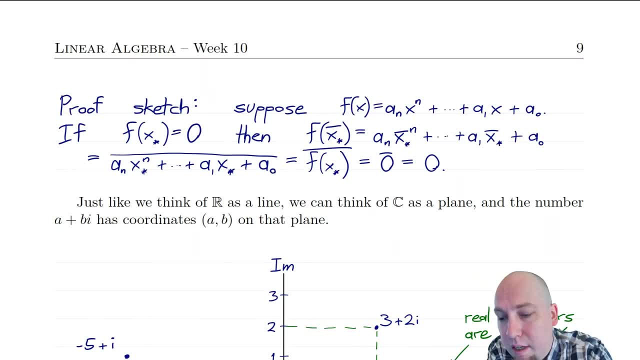 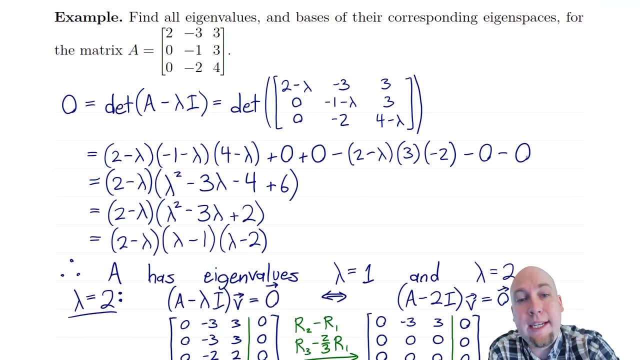 Okay, I want to go back and contrast this example with an example that we saw a few pages ago, back on page five of this week's notes. This was an example that we went through two lecture videos ago. We computed the eigenvalues of this three by three matrix as well as bases of the corresponding 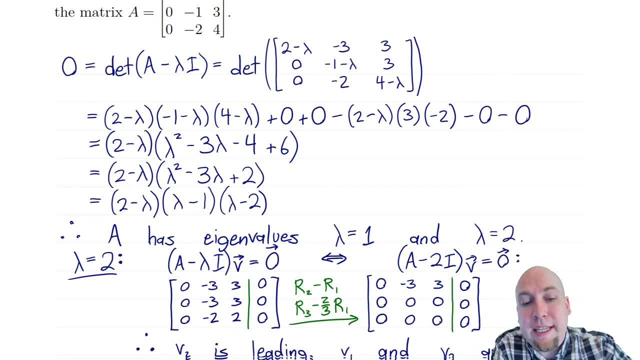 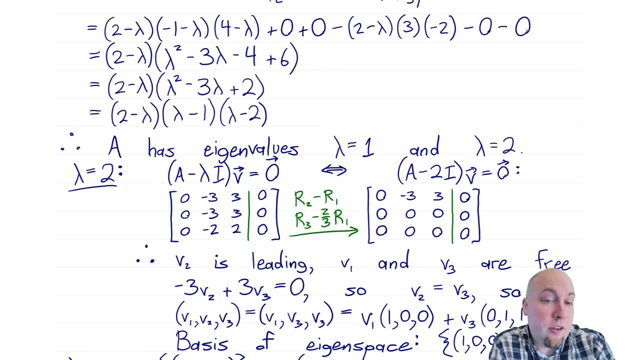 eigenspaces of this matrix. Okay, and we computed that the eigenvalues were lambda equals one and two, just like the example that we went through in today's video. Okay, and furthermore, the algebraic multiplicities were even the same. Okay, lambda equals one, with algebraic multiplicity one. 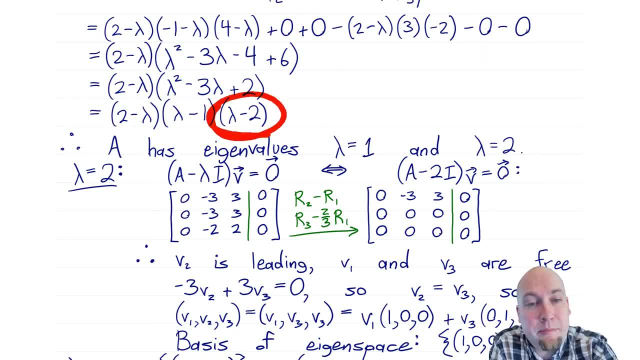 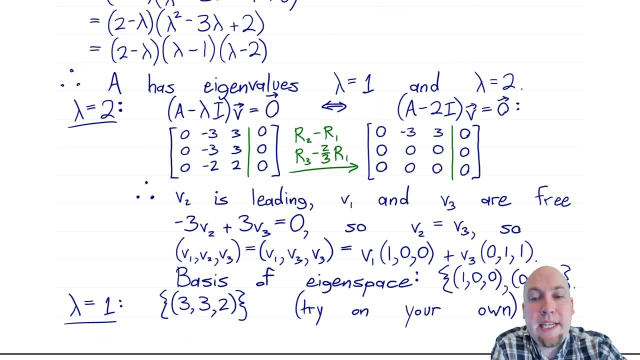 and then lambda equals two with algebraic multiplicity two, because the lambda minus two factor occurs twice here. Okay, but the geometric multiplicities are different. Okay, for lambda equals two. in the example that we went through in today's class, we found the geometric 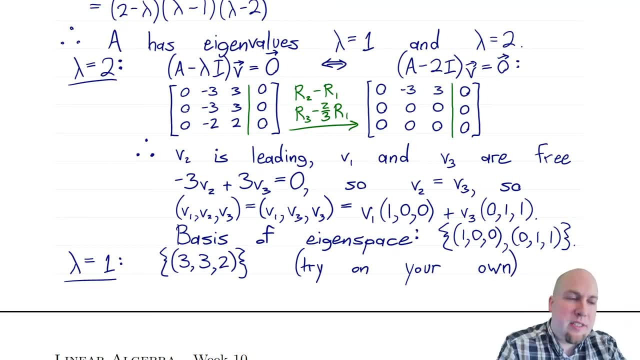 multiplicity was just one, but in this example that we saw a few pages ago, the geometric multiplicity was two, because there are two vectors in this basis of the eigenspace. So the eigenspace in this case was two-dimensional. Okay, so the geometric multiplicity is two. 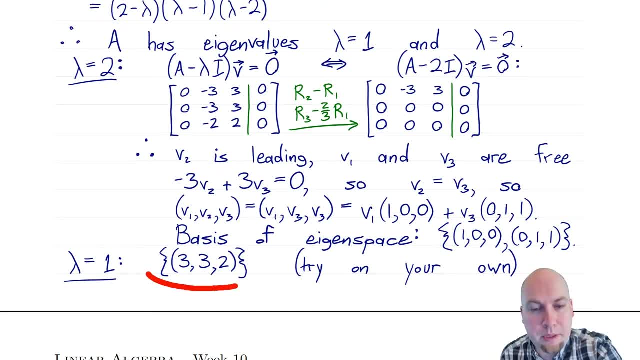 For lambda equals two. For lambda equals one. the geometric multiplicity was still just one because there's only one vector in that basis there. so the eigenspace is one-dimensional. Okay, so this maybe slightly hints at a possible theorem here. Okay, if we sort of catalog what, 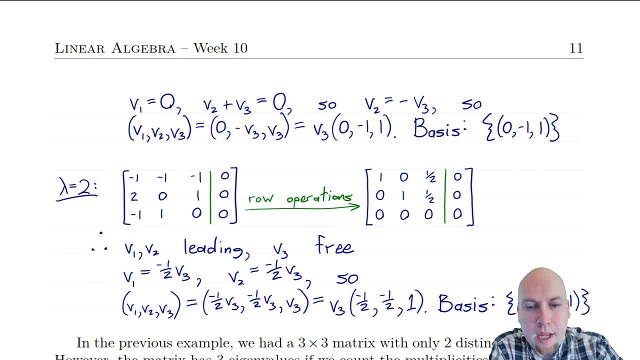 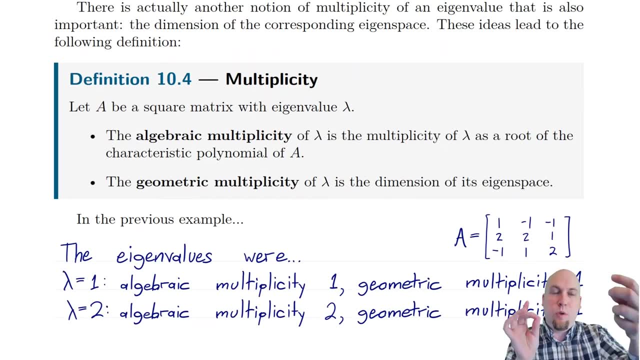 we've learned so far and sort of the examples that we've gone through, that hey, here's a three by three matrix where the algebraic multiplicities are 1 and 2, and the geometric multiplicities are one and one. and we have also seen an example where 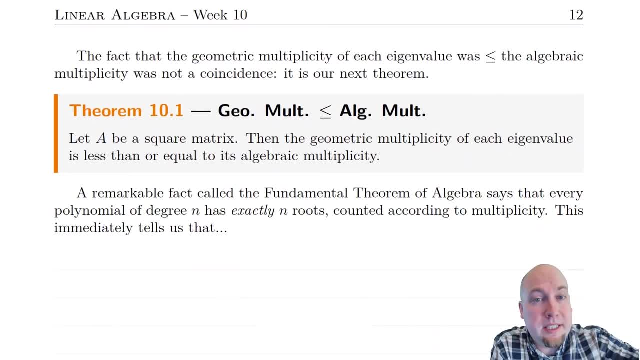 the algebraic multiplicities are 1 and 2, and the geometric multiplicities are 1 and 2.. Okay, and in every single one of those cases, geometric multiplicity isn't necessarily equal to the algebraic multiplicity, but it is always less than or equal to the algebraic multiplicity. 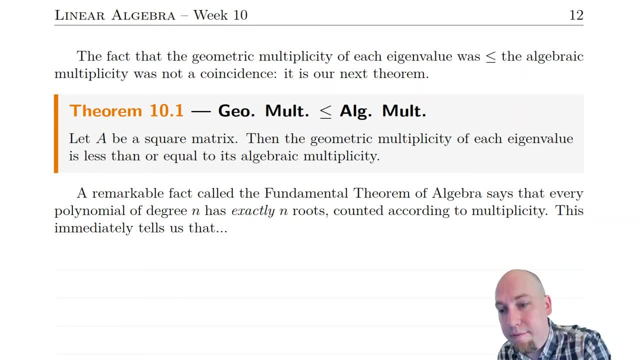 Okay, and that is true. That's true in general for every single matrix. Okay, so if you've got any old square matrix, then for every single eigenvalue of that matrix, the geometric multiplicity is gonna be less than or equal to the corresponding algebraic multiplicity. 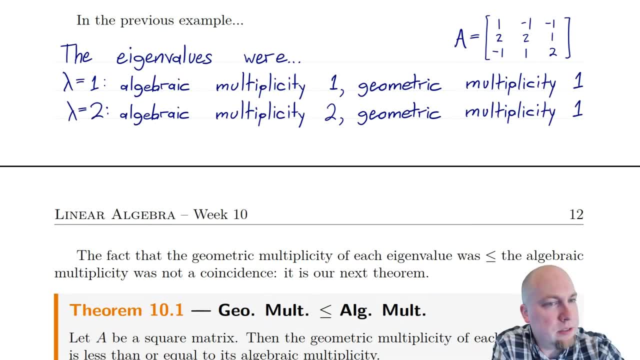 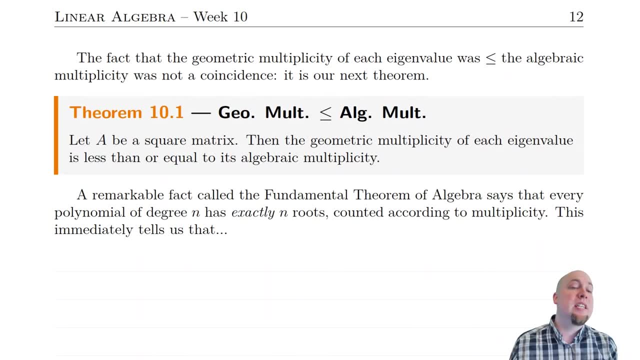 Okay. so the fact that, hey, this one is less than or equal to one, not a coincidence. The fact that this one is less than or equal to two, not a coincidence. Okay. so this is a theorem, It's proved in the textbook. 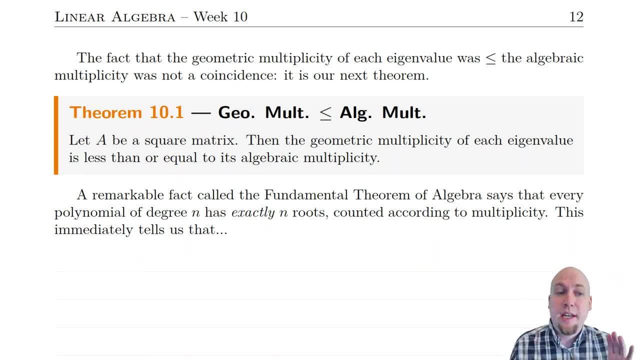 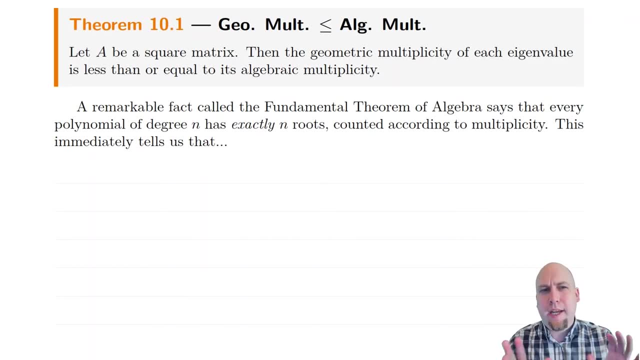 I apologize, we're gonna skip over the proof, just for time reasons. There are some things that I really want to get to at the end of this week and going into next week, and we're just running out of time to do it. Okay, there's one final polynomial-related fact. 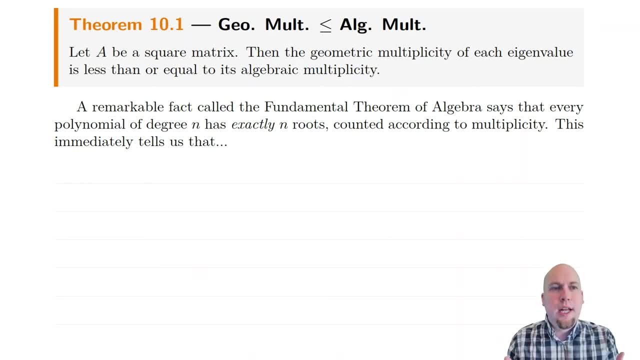 that I want to talk about and this fact. it's gonna tell us a little bit more about how eigenvalues work and, in particular, how the algebraic multiplicity of eigenvalues work. Okay, the result is called the fundamental theorem of algebra. okay, 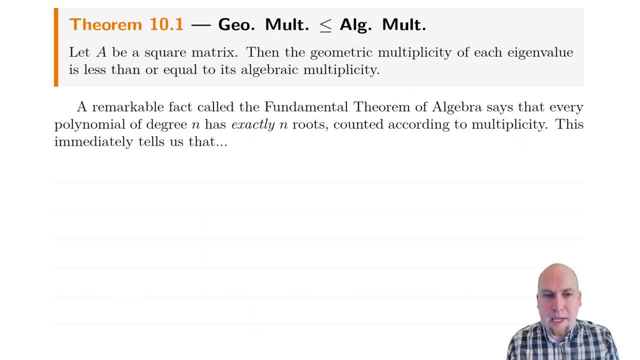 So it's a result from complex analysis. so maybe you've seen it, maybe you haven't, but what it says is: if you have any degree n, polynomial, so the highest order term is lambda to the power n. well, what it says is then that polynomial. 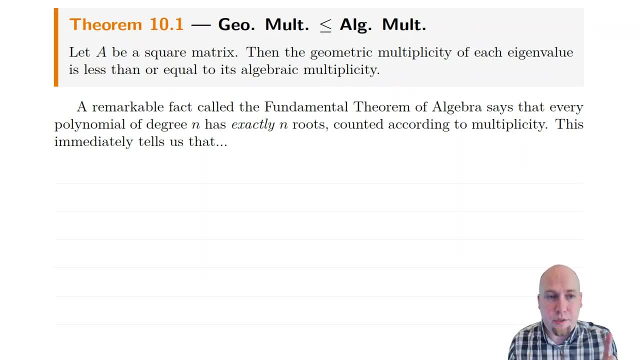 it has exactly n. Okay, as long as you do two things: As long as you allow complex numbers, okay, like your roots can be complex numbers even if the coefficients are real. and the other thing you've gotta do is you've gotta count the roots according to multiplicity. 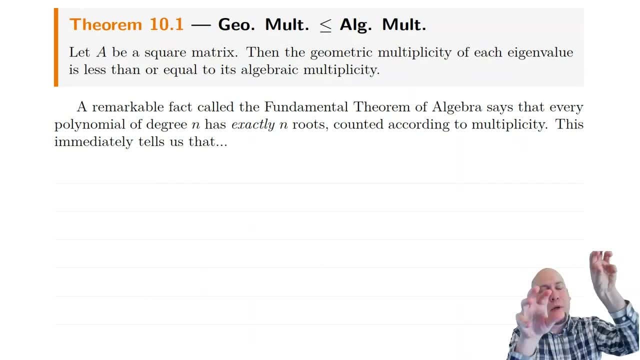 Okay, so the way that you count the roots is like you add up the exponents in the linear factors of the fully factored form of that polynomial. okay, So you're sort of counting how many times that root occurs. okay, So it's not, we're not saying. 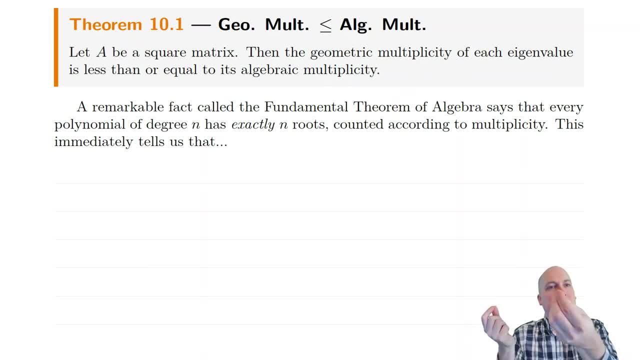 that there are exactly n distinct roots. like roots can occur multiple times, it's just you're counting up how many times they occur And if you add up all of those, hey, how many times does this one occur, and how many times does this one occur, and so on. 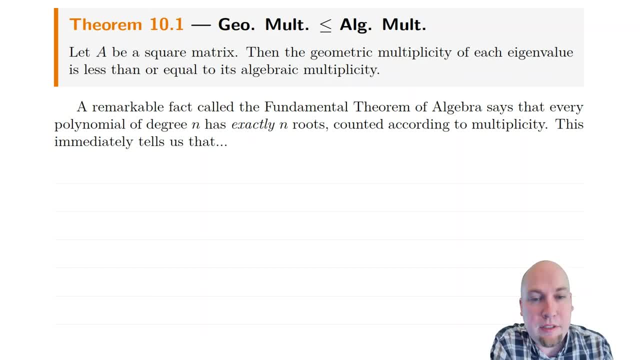 then you get exactly n. You get exactly the degree of the polynomial. Okay. and if you apply this result to the characteristic polynomial, then you get a statement about eigenvalues and algebraic multiplicities. And what that statement is is that well? 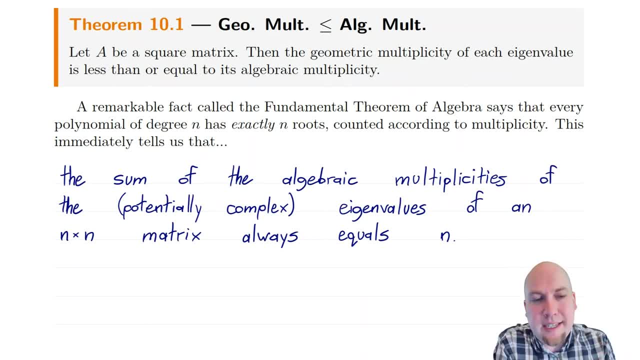 if you allow complex eigenvalues, then the sum of the algebraic multiplicities of the eigenvalues of any n by n matrix is exactly n. okay, So if you take any matrix, you compute its eigenvalues, keeping in mind that we're allowing complex eigenvalues. 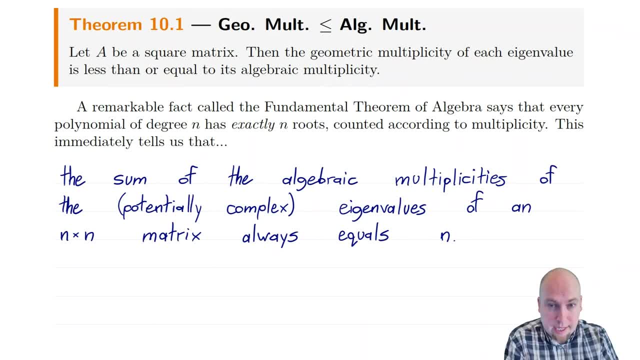 and then you compute the algebraic multiplicity of each of those eigenvalues and then you add up those algebraic multiplicities, what you will get is n. You will get the size of the matrix that you started with. Okay, and if you combine this with this previous theorem, 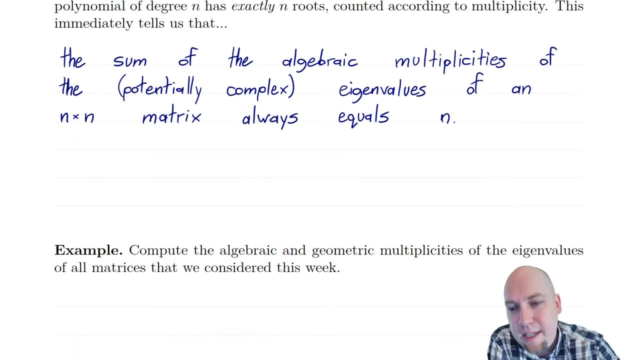 geometric multiplicity is less than or equal to algebraic multiplicity. well, we're gonna find something analogous, but a little bit weaker, for geometric multiplicities If you add up the geometric multiplicity. if you add up the geometric multiplicity. 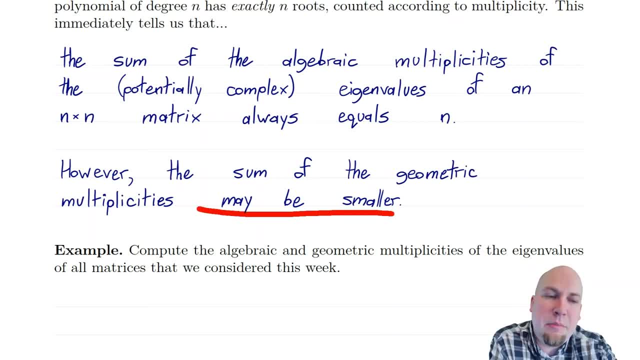 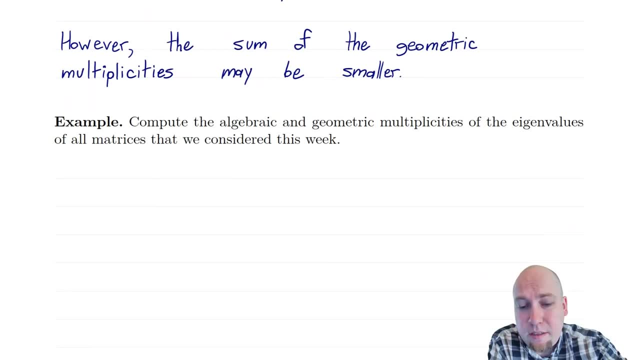 if you add up the geometric multiplicities, you might get n, but you might get something smaller as well. okay, You don't necessarily get n if you add up the geometric multiplicities. Okay, so let's just go back and remind ourselves. 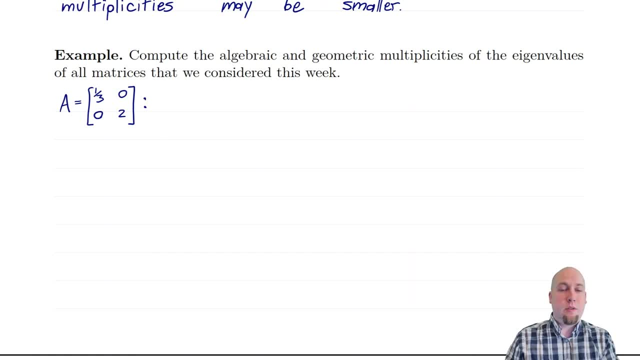 of how this works for all of the examples that we've gone through this week. okay, So all the matrices that we've seen, eigenvalues and eigenvectors for. okay, For the matrix, the diagonal matrix- that has 1, 3rd and 2 on the diagonal. 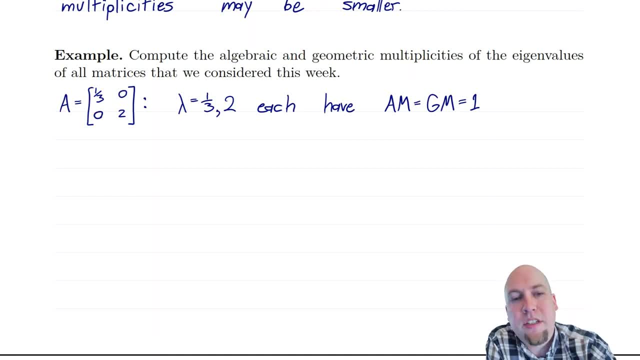 well, this matrix, the eigenvalues are exactly the 1, 3rd and the 2,. okay, We talked about how this matrix just stretches the standard basis vectors. Well, those are the corresponding eigenvectors. okay, That's just a calculation to show. 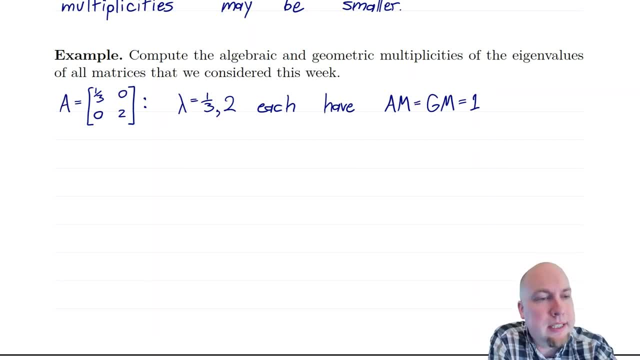 that these eigenvalues each have algebraic multiplicity and geometric multiplicity equal to 1, okay, So if I add up algebraic multiplicity is 1 plus algebraic multiplicity is 1, I get a total of 2, which yeah. 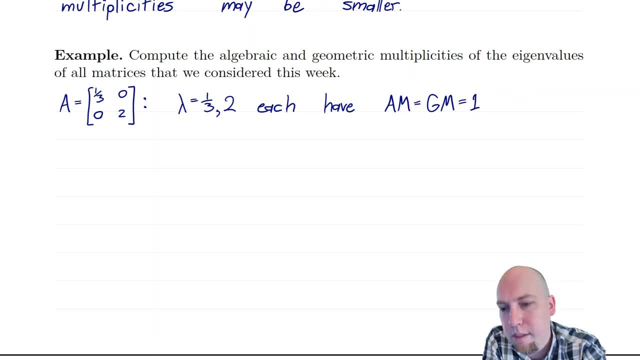 that's the size of the matrix. The matrix is 2 by 2, okay, Here's another 2 by 2 example that we looked at: this matrix: 2, 1, 1, 2.. We talked about how lambda equals 3 is 1. 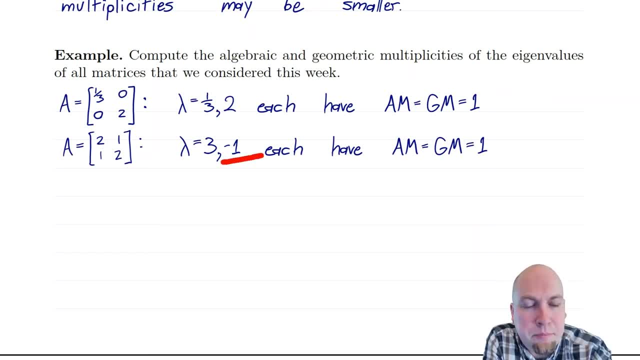 of its eigenvalues. It turns out the other eigenvalue is lambda, equals minus 1. We didn't go through that calculation, but it's something you can check now if you want to. okay, And also, it's just a calculation to show. 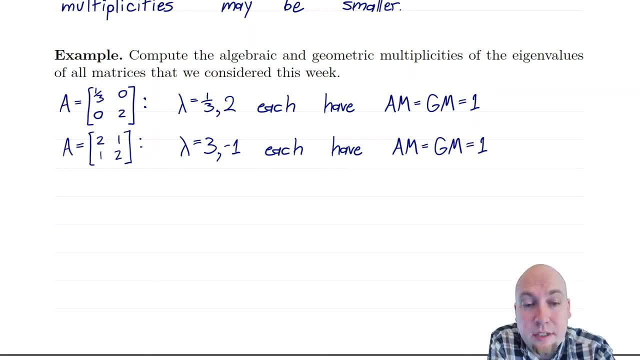 that the algebraic multiplicity of each of these eigenvalues is 1.. So again we see that, hey, 1 plus 1 equals 2, the size of the matrix Sum of the algebraic multiplicities really is 2.. 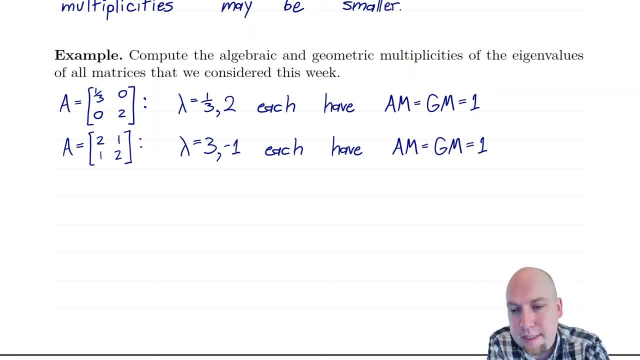 It's the size of the matrix. Geometric multiplicities are also 1 in this case. All right, another 2 by 2. example: this matrix: 1, 2,, 5,, 4, we found that this matrix is 1.. 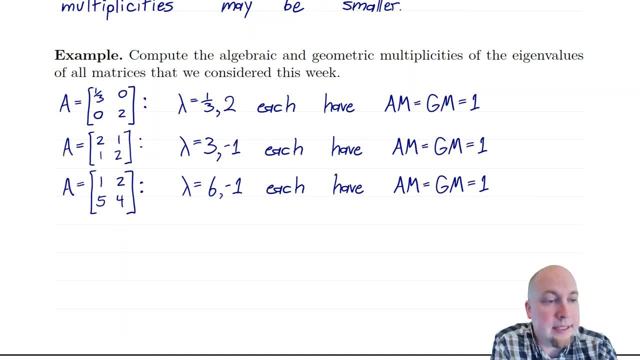 We found the eigenvalues, which were 6 and minus 1.. An exact same thing happened in this case. Algebraic and geometric multiplicities were both 1.. You add them up, you get a total of 2, the size of the matrix. 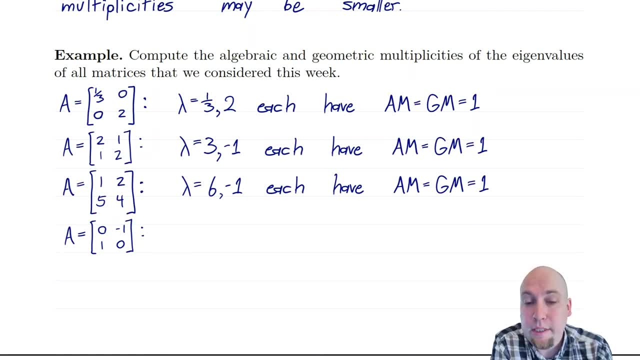 For this matrix. here our example of a matrix that does not have real eigenvalues. so 0 minus 1, 1, 0.. We found that the eigenvalues of this guy were complex. okay, they were i and minus i. 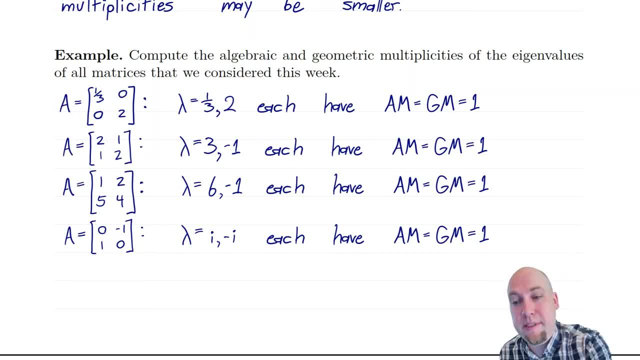 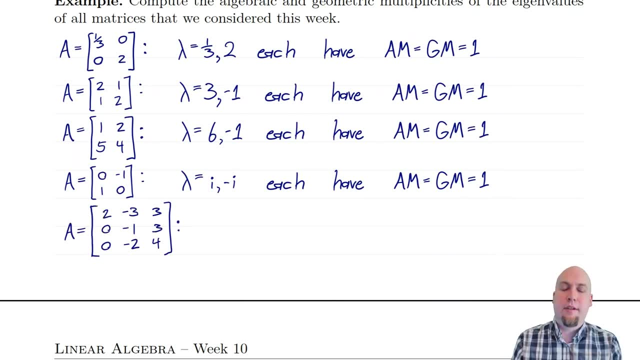 And again, they each had algebraic and geometric multiplicity equal to 1.. You add up those algebraic multiplicities, you get 2, plus 1, you get 3. You get the size of the matrix. All right, and we also went through this 3 by 3 matrix. 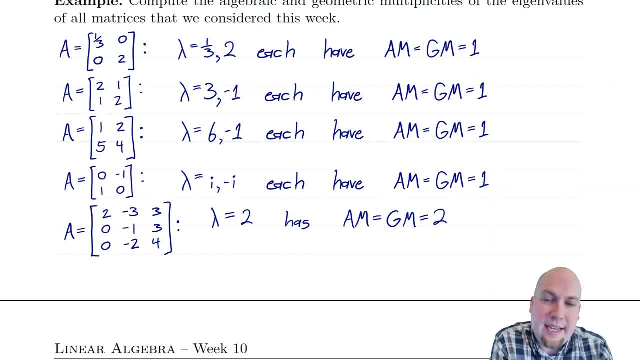 a little while ago. okay, And we found that, hey, this guy has two different eigenvalues. One of them is lambda, equals 2.. And for this one we found the algebraic multiplicity and the geometric multiplicity both equal 2.. 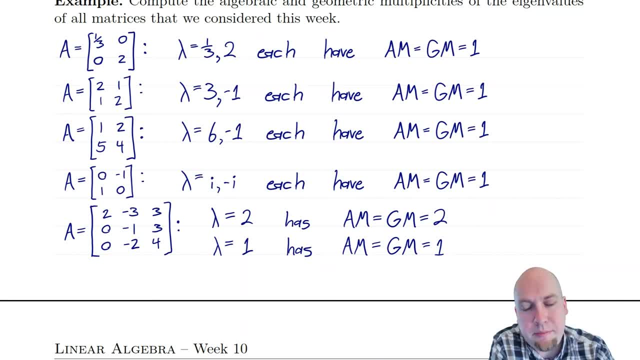 And the eigenvalue lambda equals 1, it had algebraic and geometric multiplicity equal to 1.. Okay, and if you add up the algebraic multiplicities, you do 2 plus 1, wouldn't you know it? you get 3.. 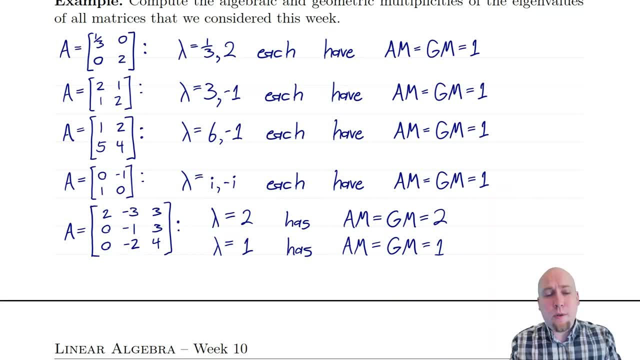 You get the size of the matrix, Okay, and that always, always, always happens. as long as you allow complex eigenvalues and as long as you sum up algebraic multiplicities, okay, The sum of the geometric multiplicities might be smaller. 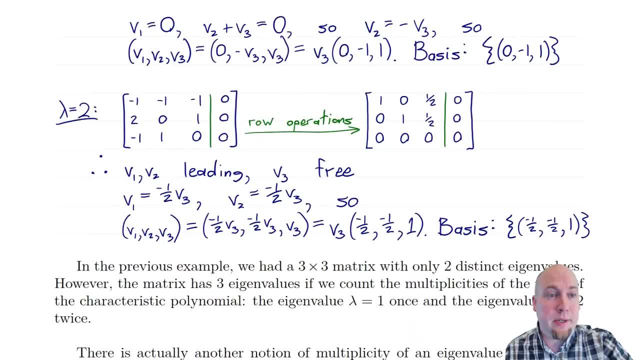 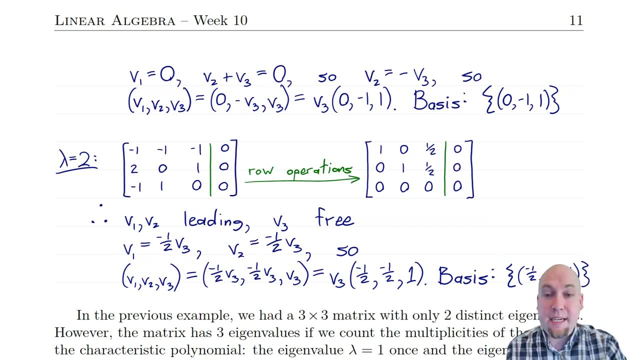 right, we saw an example of that too. Okay, that was the 3 by 3 example that we went through today. In the example that we went through today, we had geometric multiplicity 1 and geometric multiplicity 1, you add them up, you get 2.. 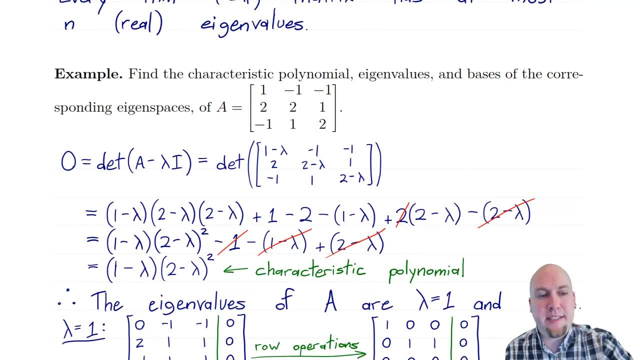 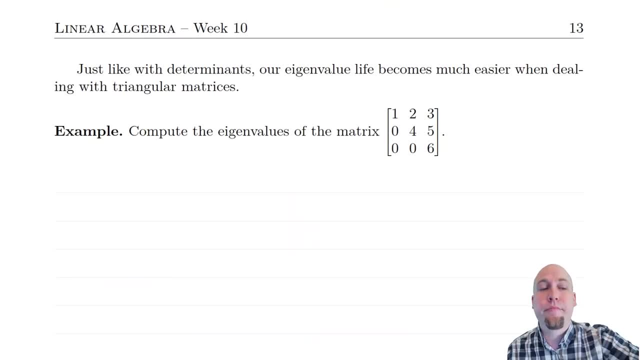 But it was a 3 by 3 matrix, okay, So the geometric multiplicities might add to something smaller than the size of the matrix. It's only the algebraic multiplicities that always add up to n. Alrighty, so that does it for facts about polynomials. 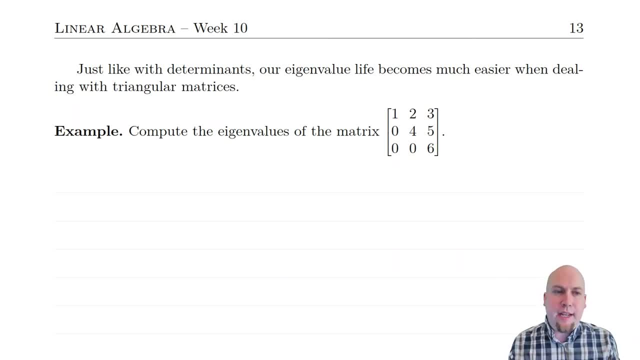 and characteristic equations. Let's go on to one final sort of special case about eigenvalues. that is a little bit easier to deal with. So this sort of special case that's nice to point out, just because it's gonna make our life easier in a lot of cases. 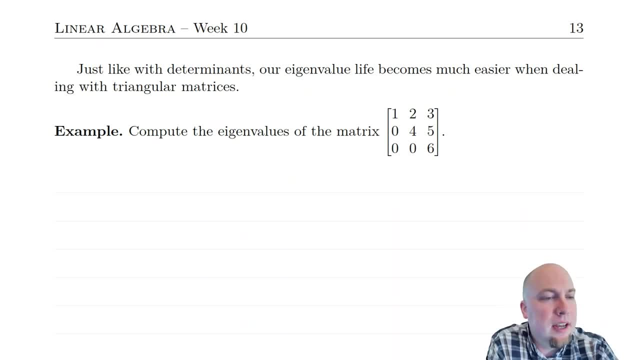 So let's think about how could we compute the eigenvalues of this matrix here. okay, So it's an upper triangular matrix. It's one, two, three- it goes down here- and then four, five and six. okay, Let's compute the eigenvalues of that matrix. 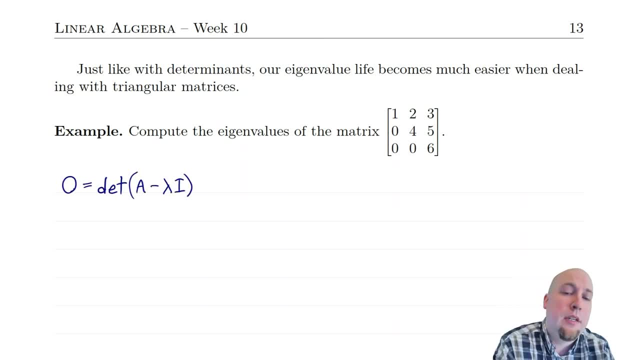 and see something that happens, And what happens is really really nice. So how do we compute the eigenvalues of that matrix? We compute determinants of A minus lambda. I set it equal to zero. okay, So that means we're subtracting lambda off the diagonal. 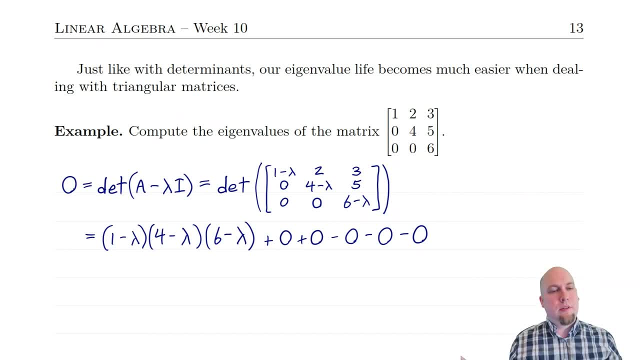 computing the determinants of that thing, And we use one of our explicit formulas. right, It's a 3 by 3 matrix, So I know how to compute that. It's forward diagonal plus next forward diagonal, Oh, but it has a zero in it. 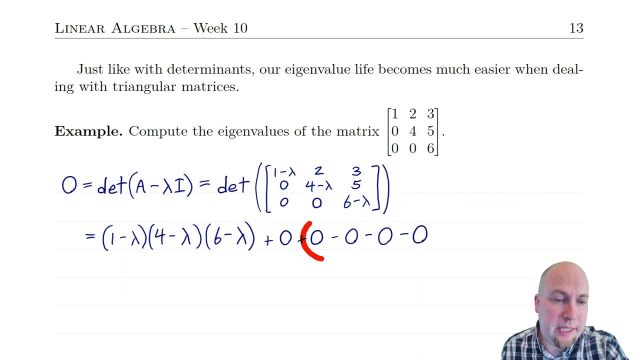 So that's a zero. And then plus next forward diagonal, Which has a zero in it, So that's a zero. And all of the backward diagonals have zeros in them, right? They all hit at least one of these zeros in the bottom left corner. 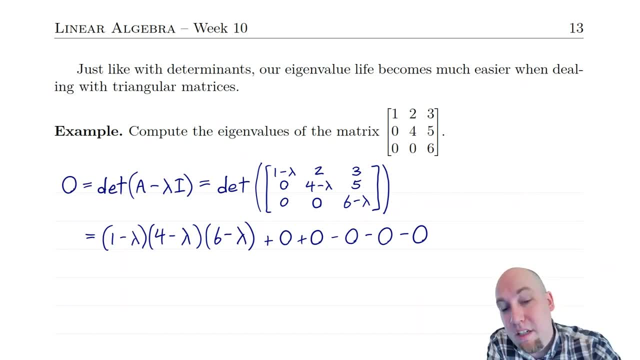 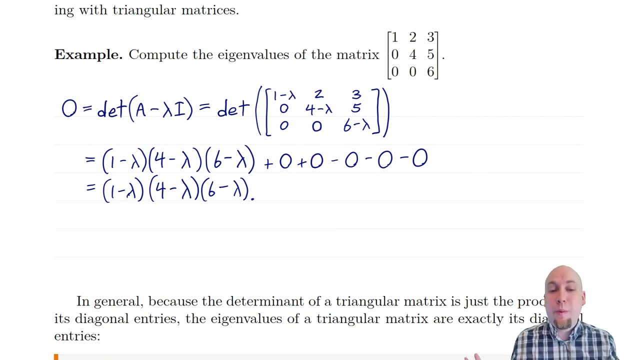 So the only term in this explicit formula that does not die off because of a zero is the one coming from the main diagonal. okay, So our characteristic polynomial. we don't need to do any work whatsoever to factor it, It's already factored for us. 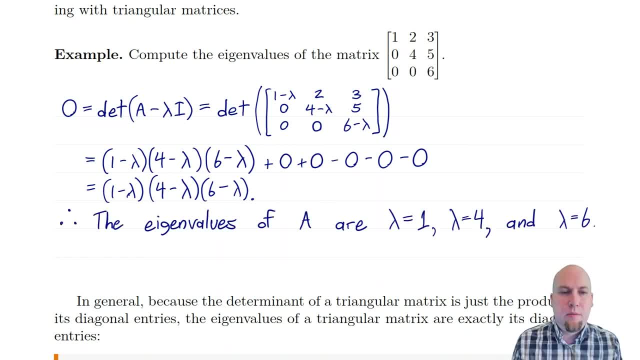 So we can see right away: hey, what are the roots of that polynomial? Well, they're just one and four and six. So those are the eigenvalues of the matrix, okay, And if you squint really hard at that, you're gonna notice that, hey, one, four and six. 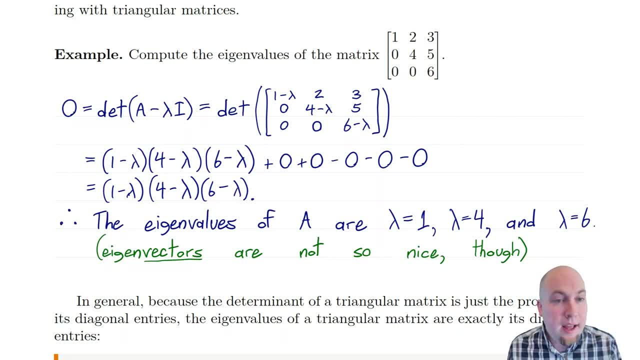 those are exactly the diagonal entries there, right? That's not a coincidence, okay, That always, always happens. as long as your matrix is triangular, either upper triangular or lower triangular- Then the eigenvalues of your matrix easy, easy, easy to find out. 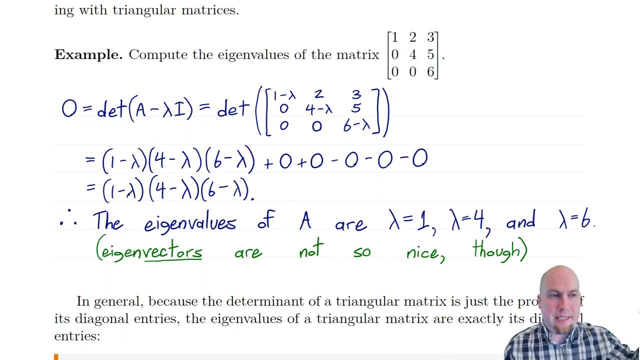 They're just the diagonal entries, okay. The eigenvectors, though. don't expect a nice roll for those. The eigenvectors still might be ugly, okay, So that's the diagonal entries. So we're just gonna state this as a theorem, okay. 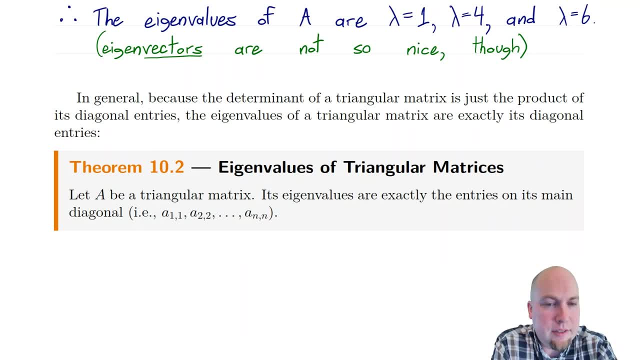 because it's gonna be useful for us going forward. okay, So if you have a triangular matrix- so upper triangular, like in this example, or lower triangular is also fine- then its eigenvalues are gonna be exactly its diagonal entries. So A11,, A22, up to ANN, always, always, always. 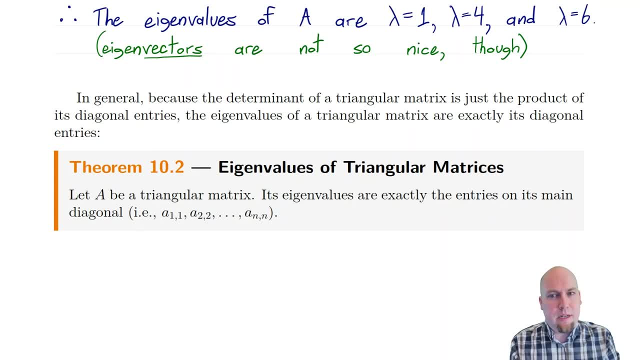 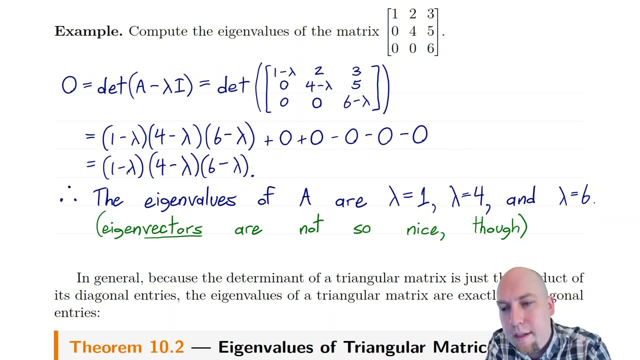 And where's that come from? Well, it comes from the fact that- well, I mean the determinants of a triangular matrix is just the product of the diagonal entries. right, That's the theorem that we saw last week. okay.